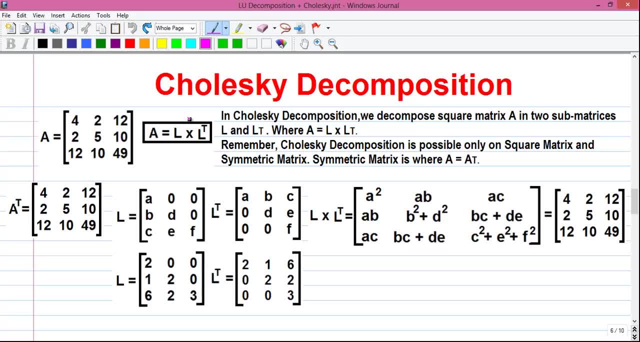 below, So check them out. Today in this video I will tell you how to do the Cholesky decomposition of a 3 cross, 3 square matrix. I have also four videos on the LU decomposition, another decomposition technique. Link to all of: 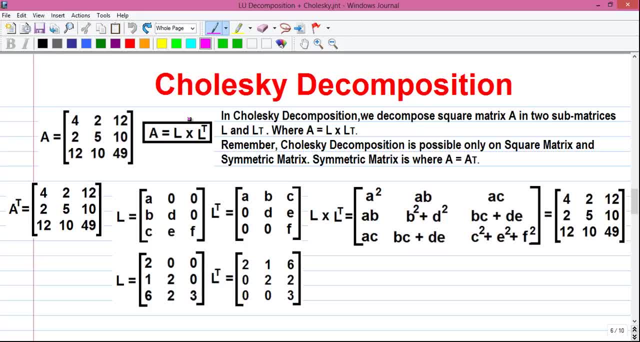 them is given in the video description below. So let's start today's video. So, before we start with the calculation, let me tell you some basics. This is called row 1, this is row 2 and this is row 3.. Similarly, this is called the column 1,. 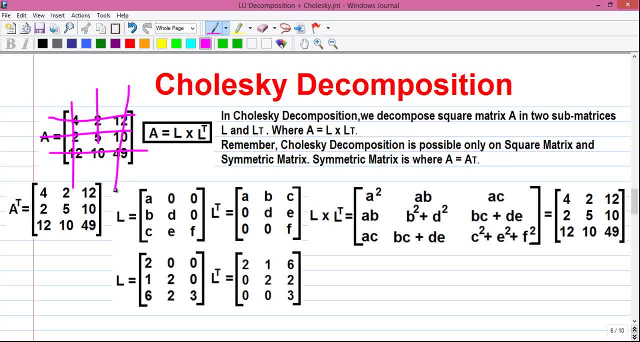 this is column 2 and this is column 3.. Now the basics of Cholesky decomposition. In Cholesky decomposition we decompose a square matrix a into submatrices L and LT, or transpose of L, where the matrix a is equals to L, into transpose of L That I have written here. 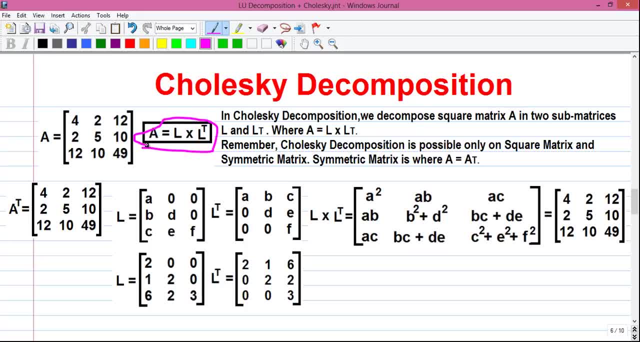 A is equals to L- into transpose of L where L is a lower triangular matrix. This is the standard form of L, where the values or numerical values are there in the lower triangle and the upper triangular values are all 0, and this is the transpose of L, or LT for short. So here the first row of L is A00.. So we will. 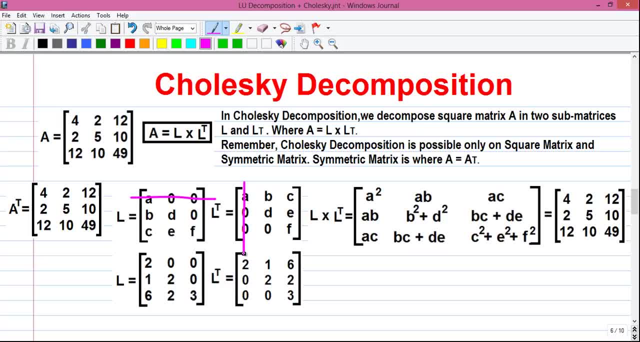 write that as column 1 in LT A00.. Similarly, the row 2 of L will become the column 2 of LT And the row 3 of L will become the column 3 of LT. So that is, by writing rows into columns. 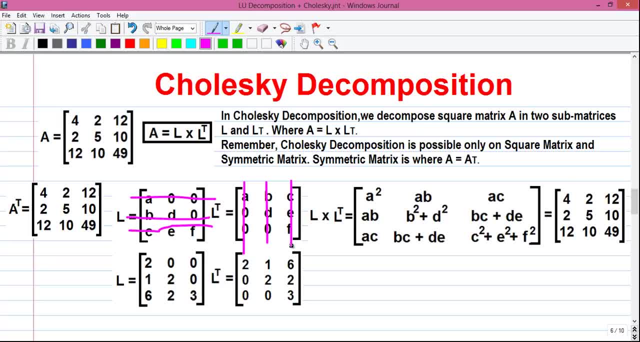 you will get the transpose of R: square matrix. Remember the Chomsky: decomposition is possible only with the square matrix and with symmetric matrix. Square matrix means where the number of rows is equal to the number of columns. So here our original matrix. A is a square matrix. 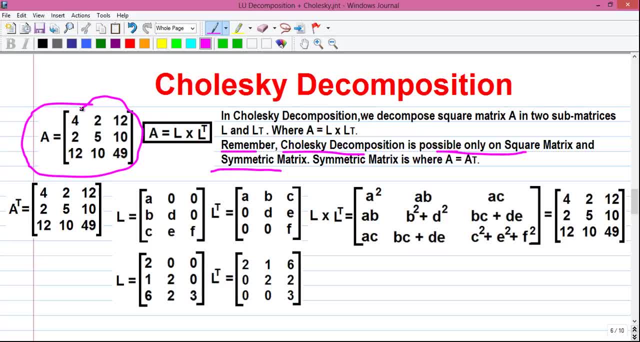 Since the number of rows is equal to number of columns is equal to 3, both are same And the Chomsky decomposition is possible with the symmetric matrix. The symmetric matrix means where the matrix A is equal to the transpose of matrix A. That means the matrix and its transpose. 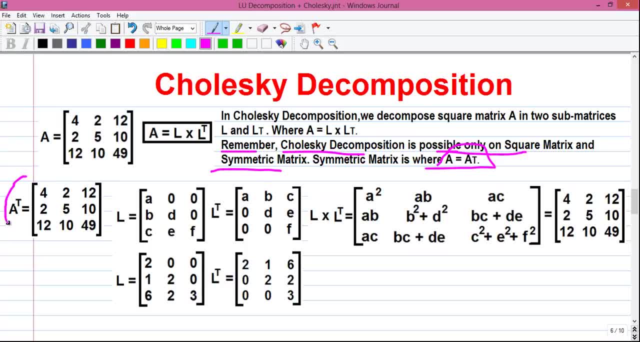 both are equal, So that I have written here: This is the transpose of original matrix A, This is the structure of the matrix A. So here I will write this whole thing. So, from the matrix A to the transpose of matrix B, this is the right answer. So until and until we get the transpose of matrix A, 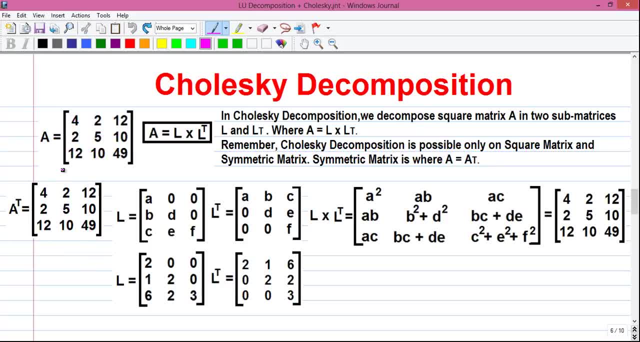 both are same. So the Chomsky decomposition of A is possible. This check you have to perform before you start the next step, So I will do a qualified check first. So I will write that in this way. Okay, 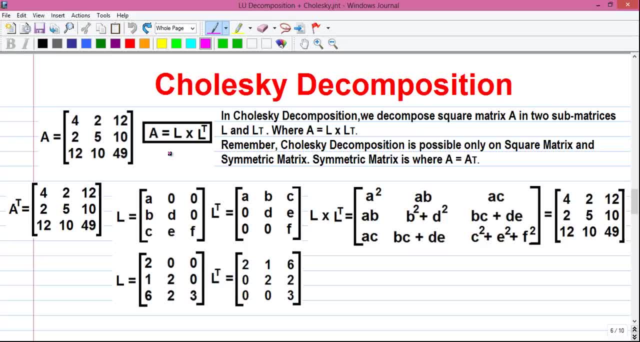 So this is a graph. This is a graph doing the Cholsky decomposition. Next we will find out the sub matrix L and the sub matrix LT. For that we'll use this property. We know the matrix A is equal to L into LT. So we know the standard form of L and by transposing it we'll. 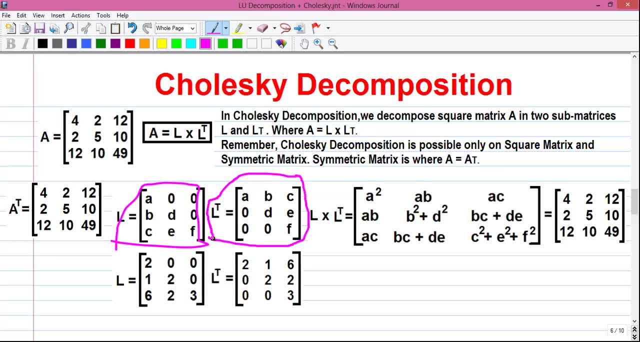 get the standard form of LT. and now we'll multiply these two matrices. I hope you know the matrix multiplication. if you don't, don't worry, I will tell it to you. a into a is a square written here. plus 0 into 0, plus 0 into 0, so that is. 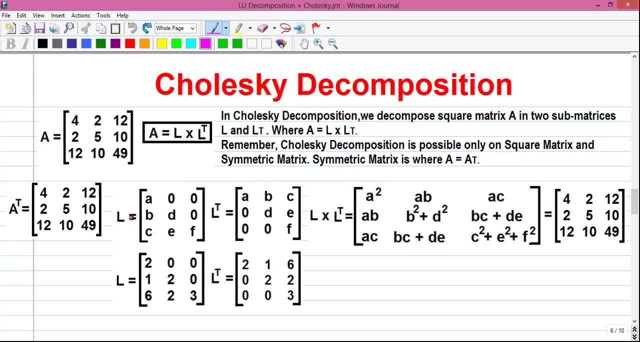 equal to a square written here. Next, we will multiply the row 2 of L with the column 1 of LT, So b into A plus b into A, and there is the dates, the times of 7 with an actual, of The 4 with 2 of 0.. 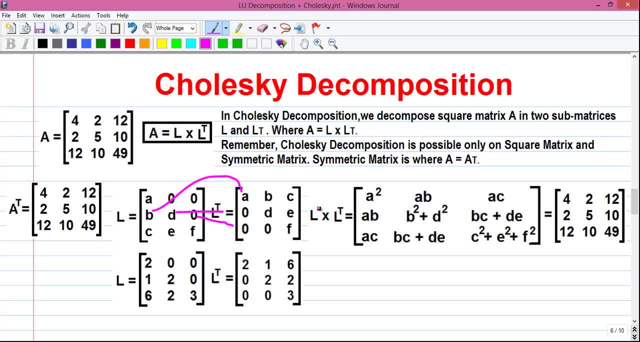 Next we multiply the row 2 of L with the column 1 of LT and there is the units of d into 0 plus 0 into 0. that's equals to a b written here. Next we will multiply the row 3 of L with the column 1 of LT. 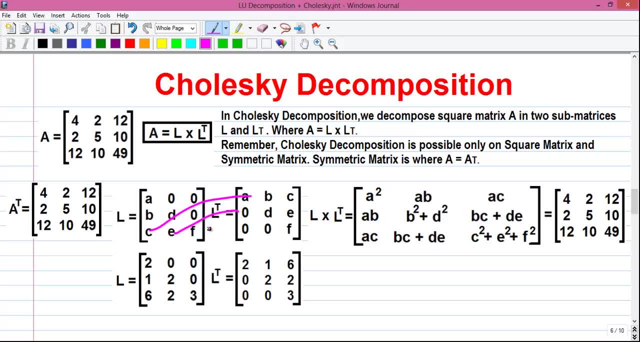 So c into a plus e into 0 plus f into 0, that's equals to a into c or ac written here. Next we will multiply the row 1, row 2 and row 3 of L with the column 2 of LT. 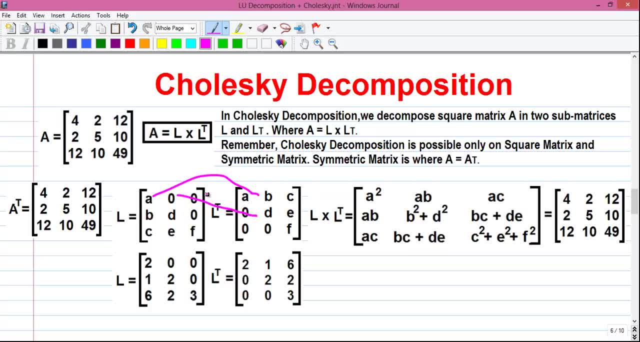 So a into b plus 0 into d plus 0 into 0, that's equals to a b written here. Next we will multiply row 2 of L with column 2 of LT. that's equals to a b written here. So b into b plus d into d plus 0 into 0, that's equals to b square plus d, square written here. 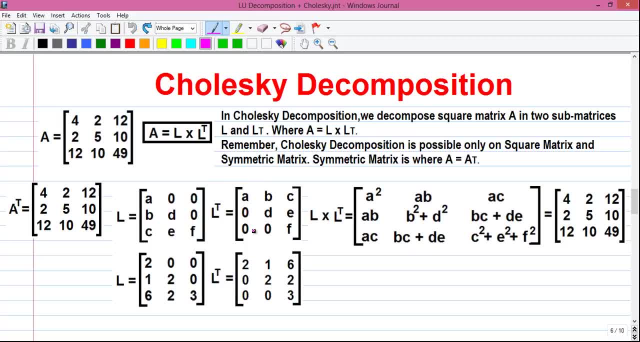 Next we will multiply row 3 of L with the column 2 of LT. that's equals to c into b plus e, into d plus f into 0. that's equals to bc plus de. that's written here. So next we will multiply the row 1, row 2 and row 3 of L with the column 3 of LT. 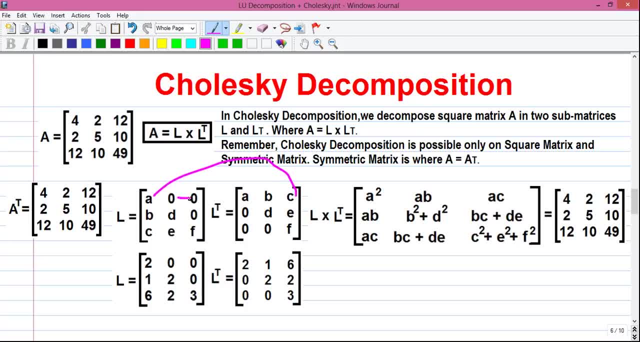 So next, a into c plus 0 into e plus 0 into f, that's equals to a into c or ac written here. Next we will multiply row 2 of L with the column 3 of LT. Next we will multiply row 3 of L with the column 3 of LT. 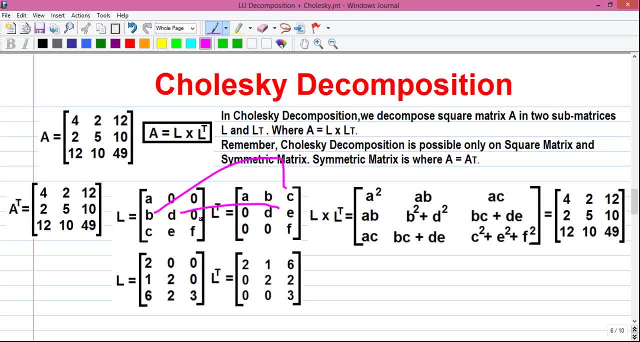 So let's do it: c into c plus e into e plus f into f, that's equals to a. c into c plus d into e plus 0 into f, that's equals to bc plus de written here. Next we will multiply row 3 of L with the column 3 of LT. 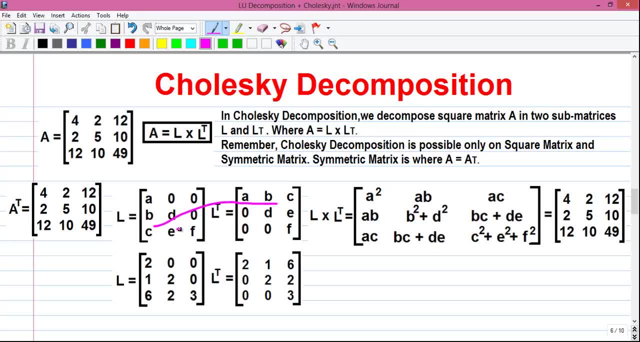 So let's do it c into c plus e into e plus f into f, that's equals to c square plus e square plus f square. So let's do it c into c plus e into f, that's equals to bc plus e plus f, that's equals to a c into c plus e plus f, that's equals to bc plus b. 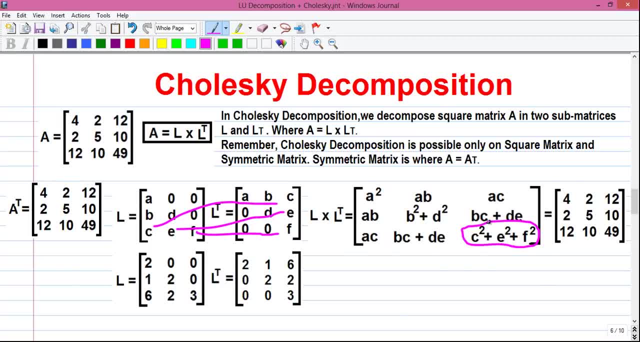 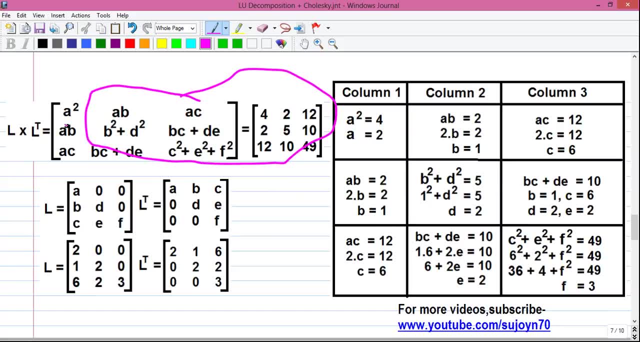 That's written here. Next we will relate these two matrices to get the values for a, b, c, d, e and f. So we will make a table like this and do the calculation. a square is equals to 4.. 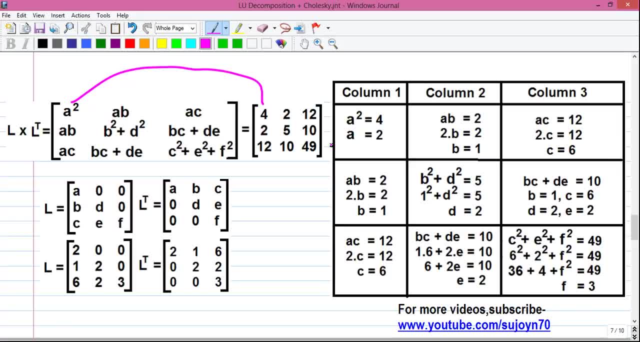 So a is root of 4 or 2.. That's written here. Next, a, b is equals to 2.. a is 2, so a, b or 2 into b is equal to 2, so b is equal to 1. written here. 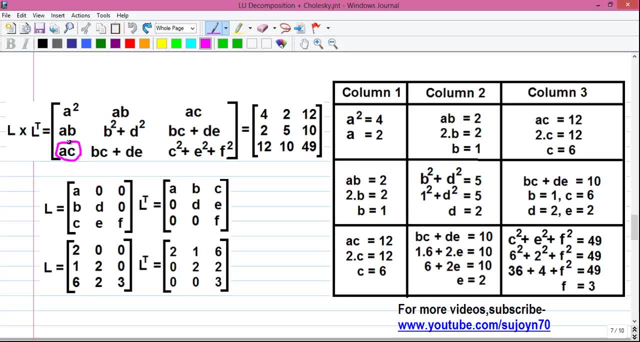 a c is equal to 12. we know a is 2, so a c is equal to 12. a is 2, so c is equal to 12 by 2 or 6. so column 1 is complete. next we will calculate column 2. for that we will compare the column 2 of. 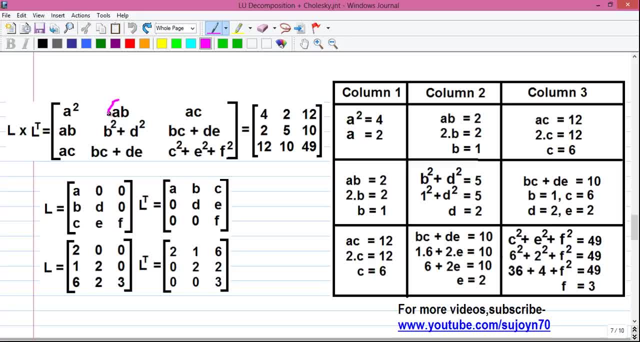 this matrix with the column 2 of a. so a, b is equal to 2. so you have already calculated the a b, so we don't need to calculate it again. we know the values for a and b. next, b square plus d square is equal to. 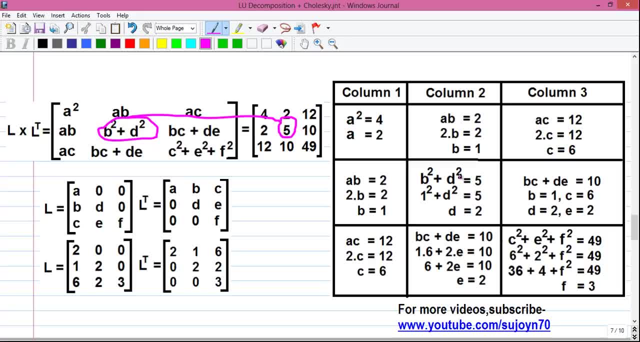 number 5. so we know the b equals to 1. so we can write: 1 square plus d square is equal to 5, or d square is equal to 5 minus 1 square, that is equal to 4. so if d square is 4, then d is equal to 2, next b, c plus d is equal to 10. 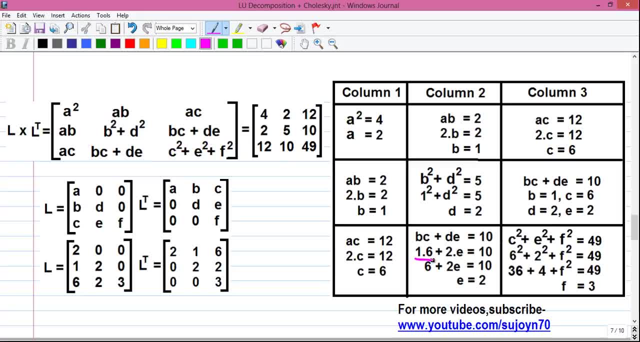 so b into c is 1 into 6 plus d into e, that is, 2 into e is equal to 10. or we can write: 6 plus 2e is equal to 10, or 2e is equal to 10 minus 6, 4. so if 2e is 4, then e is equals to 2. 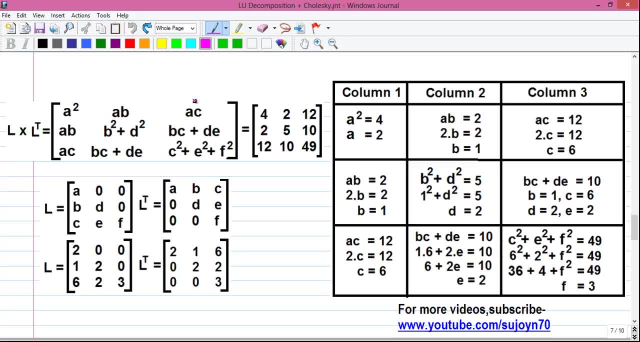 so column 2 is done. next we'll calculate the column 3 with comparing the column 3 of this matrix of A. So AC is equal to 12.. So we have already calculated AC here, So we do not need to. 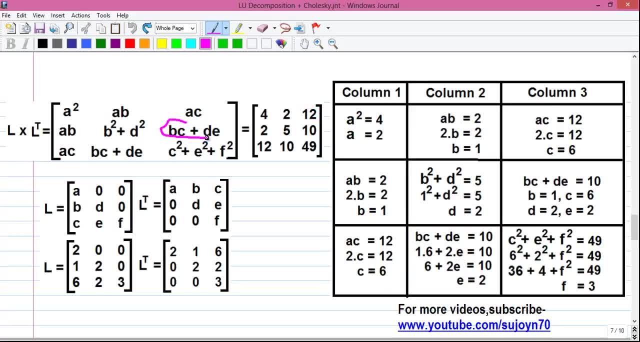 calculate AC again Next. BC plus DE is equal to 10.. So we have already calculated the BC plus DE value here. So we know the values for B, C, D and E. Finally, you have to calculate the C square plus E square plus F square, which is equal to 49.. So we know C is 6.. So we 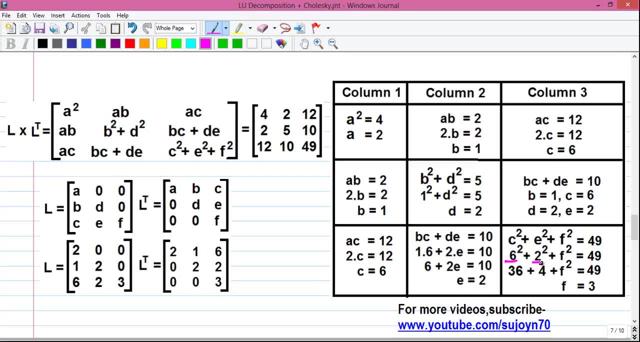 can write 6 square. We know E is 2.. So we can write E square or 2 square plus F square is equal to 49.. So C square is 36 plus 2 square is 4 plus F square is equal to 49.. So if we transfer, 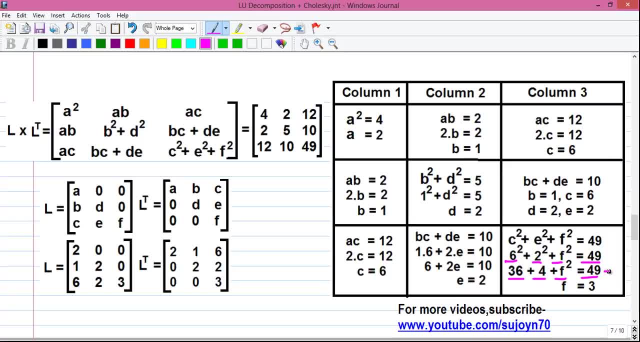 the 36 plus 4, 40 to the right hand side, we will get 49 minus 40. That is equal to 9.. So if F square is 9, then F is equal to root of 9 or F is equal to 3.. So from this, 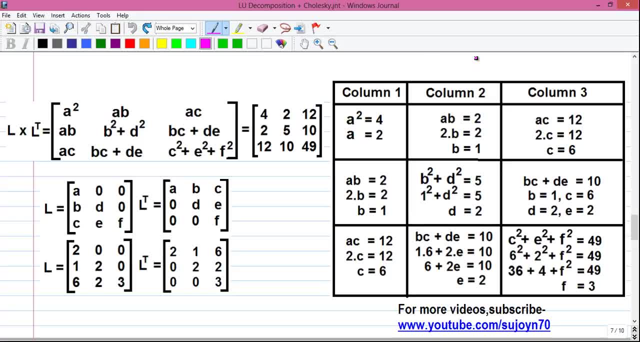 table. we have obtained the values for A, B, C, D and E. Now we will put those values into the standard form of L to get the actual L-matrix. So we know: H, 2 written here. B is 1. written here. C is 6 written here. D is 2, written here E. is 2 written here, D is 4 written here, E is 4 written here 5, and D is 5 written here And, of course, d is 1, 1. he has to情况 Hardly standing with C 2.. Please consider the figures. 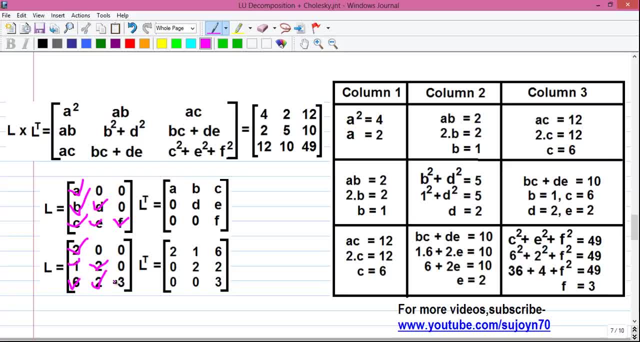 So consider the figures called C, D. This express the respect for a value in C form after I write, and f is 3 written here, and all other values are 0 as it is. so we have obtained the matrix L. now we will transpose it. we will write the row 1 of L as column 1 of LT. so 2: 0, 0 written column. 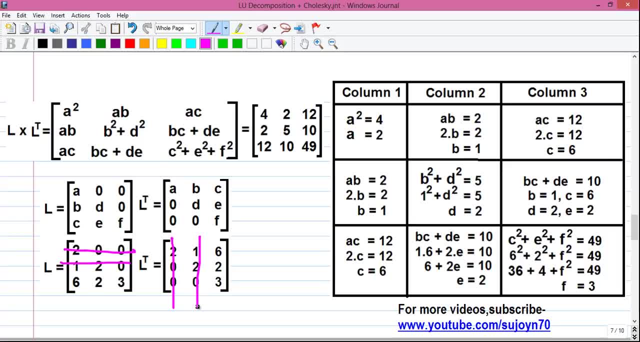 wise: 1 to 0 written column wise and 6 to 3 written column wise. that is our required LT matrix. so you have successfully decomposed the matrix a into 2 summation: L and LT. now if we multiply the L into LT, you will get the original matrix A. now I'll show you the proof of L into LT using the cation. 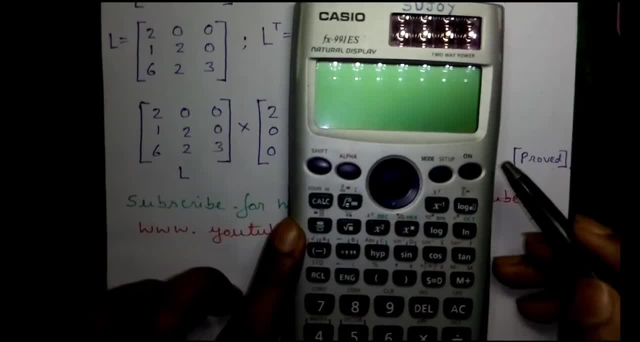 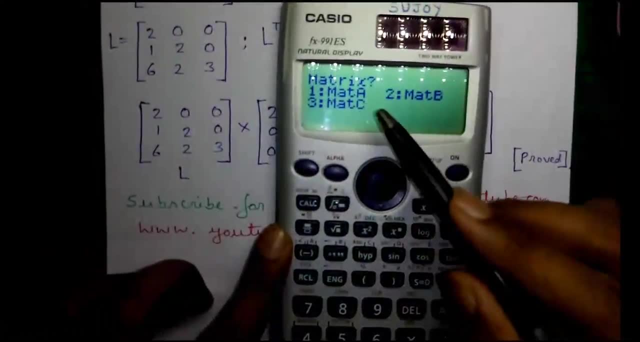 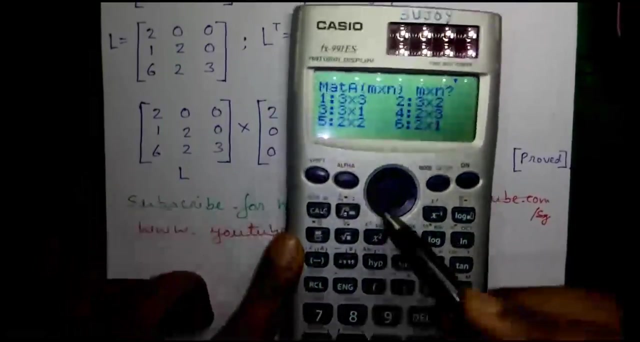 of X nanoią in the formula or the productstockİye that we have called in hyperbolic set. so C6 is, Yes, scientific calculator. So to use the matrix mode, go to the matrix mode by pressing mode 6 for matrix, 1 for matrix A, 2 for matrix B and 3 for matrix C. So first we will enter matrix A, So press 1.. 1 for 3, cross 3 matrix And now enter the data. 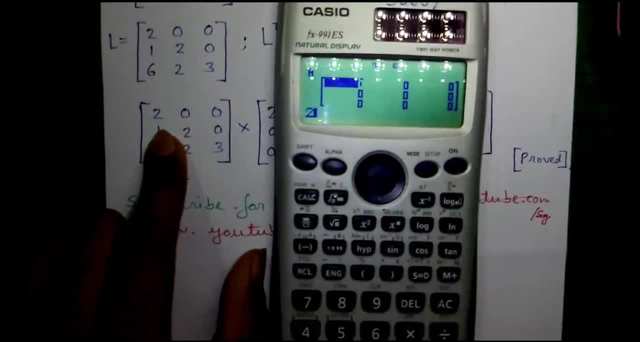 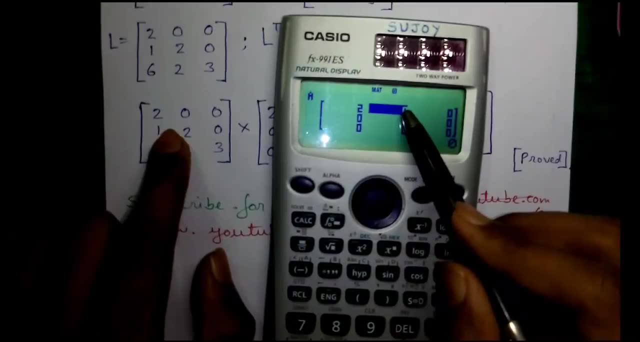 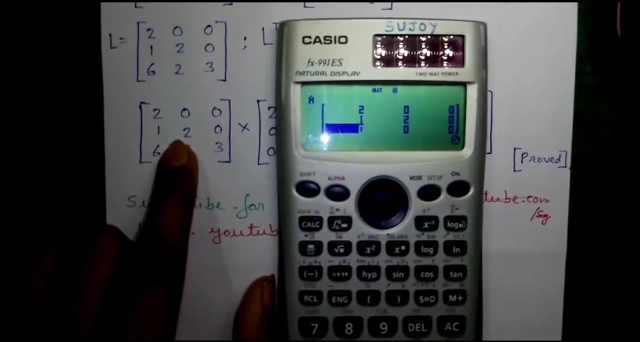 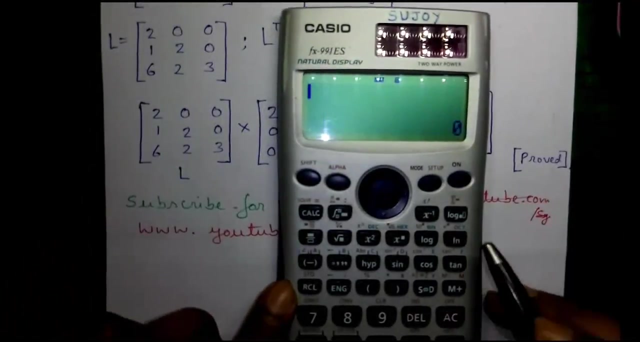 So to enter the data type in the value and press equals to button, So 2 is entered And the cursor will automatically move to the next field And keep entering the value and press equals to, So A is entered. Next press A to clear screen And to enter B, press shift 4.. 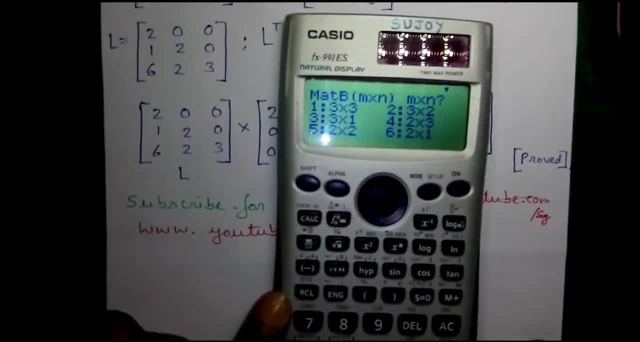 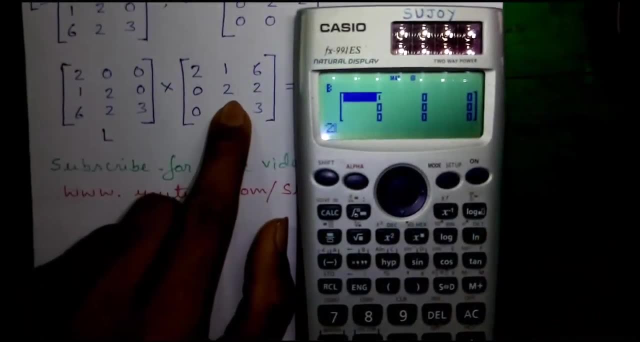 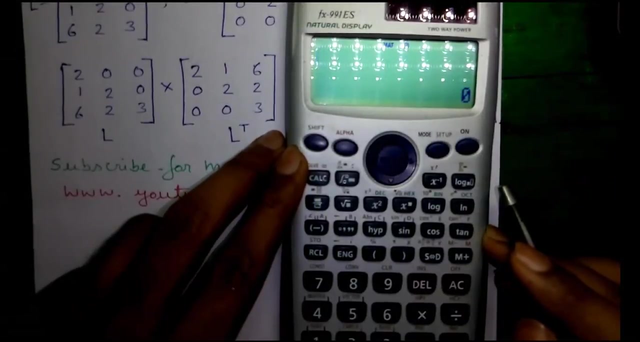 2 for data and 2 for matrix B And 1 for 3 cross 3 matrix. And now we will enter L T as matrix B, And now we will multiply the matrix A into matrix B, That is L into L T, So to get matrix A, press shift 4.. 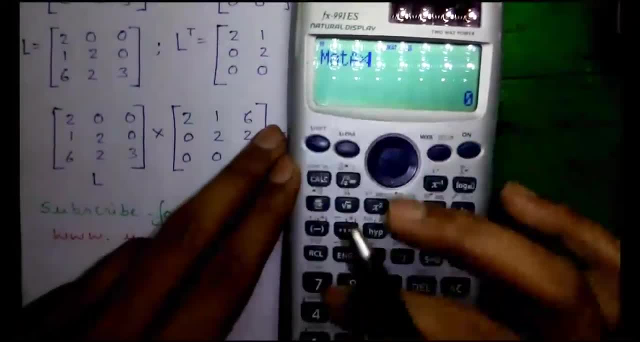 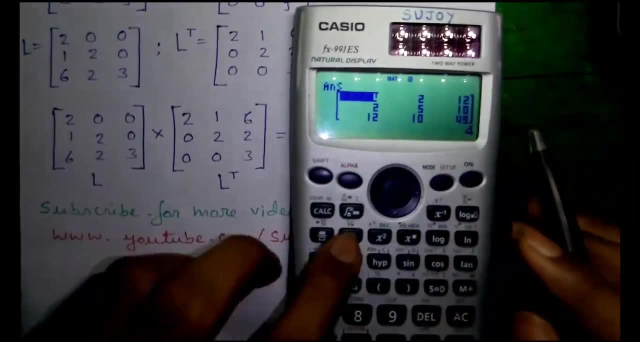 3 for matrix B, And now we will enter L T as matrix B, And now we will multiply the matrix A into matrix B, That is, L into L T. 4 for matrix A Into shift 4.. 4 for matrix B And press equals to: You will get the original matrix A. 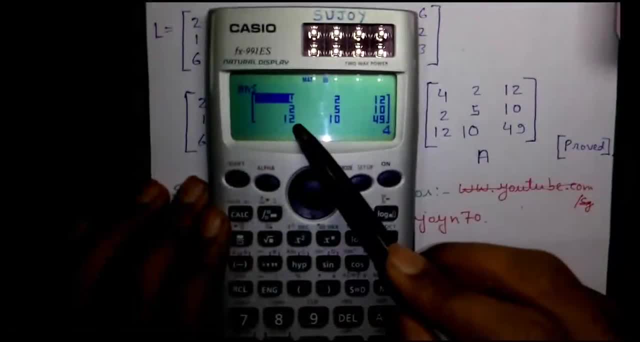 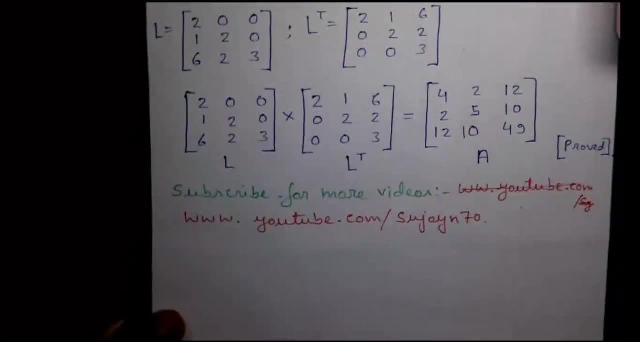 4, 2, 12, 2, 5, 10, 12, 10 and 49.. Isn't it cool? So this is my another video on computer aided teaching, or CAT. How was the video? Let me know in the comments below.